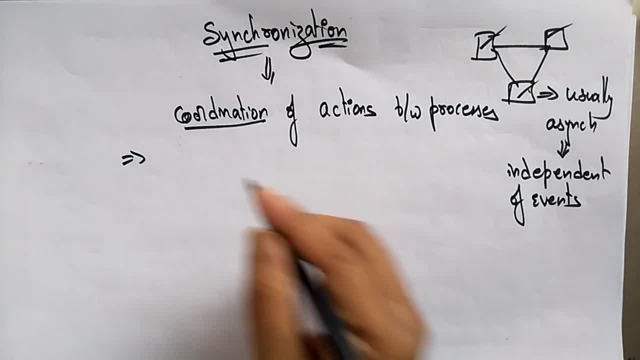 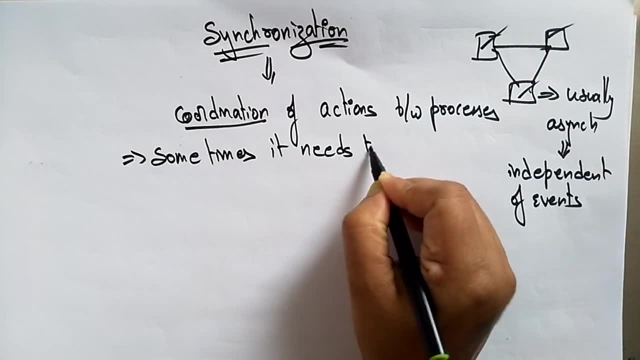 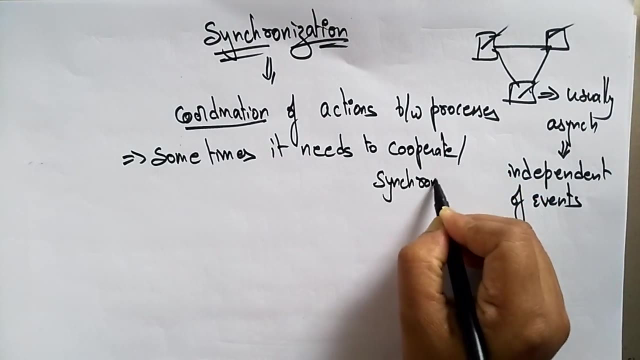 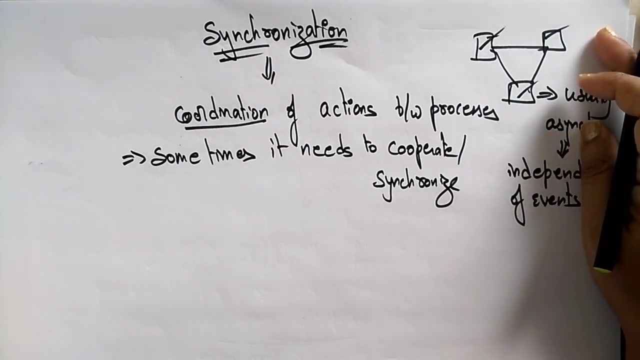 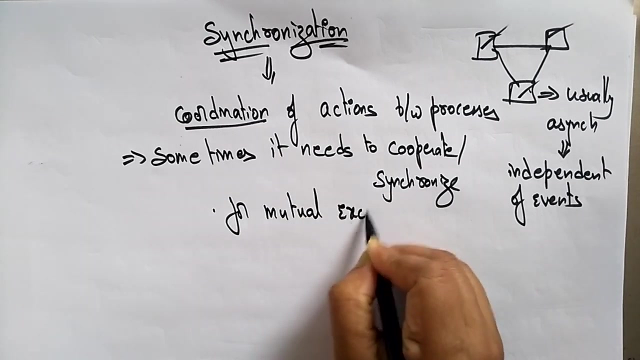 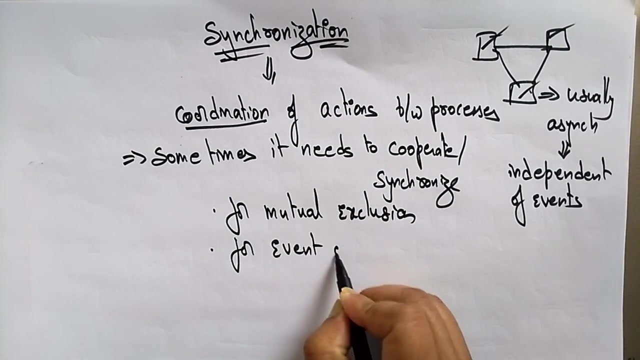 so sometimes it's need to cooperate and synchronize. sometimes it needs to cooperate or synchronize. so for what? why we need cooperation between the process and why we need to synchronize the process. because for mutual exclusion, for mutual exclusion and for event ordering. for event ordering, so here the event ordering mean, suppose some message x from process p. 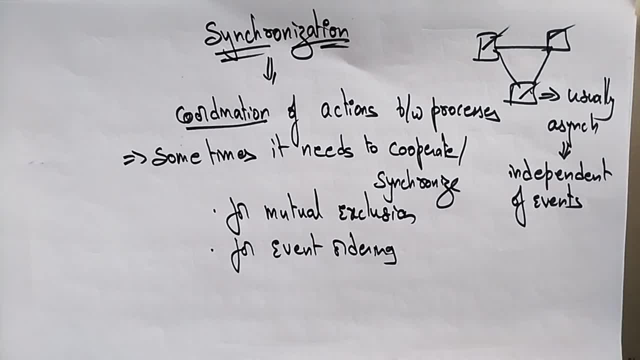 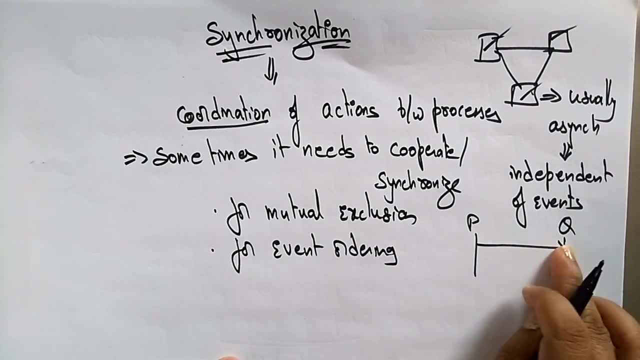 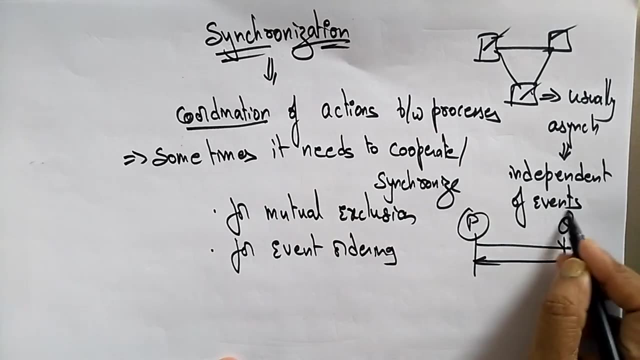 send, or be send before or after the message. y from process q means when the message has to be sent from to p, from p to q and from q to p, so how the message has to be transferred. so So there should be a cooperation between the process P and Q so that the data cannot be lost. 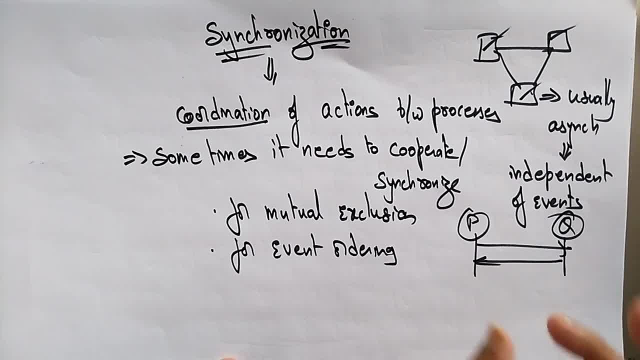 and if there is a mutual understanding between the process, then it is the time will be reduced, means you can access the data very quickly without the loss of data. So sometimes it needs to cooperate or synchronize the process for the mutual exclusions and for event ordering. So here 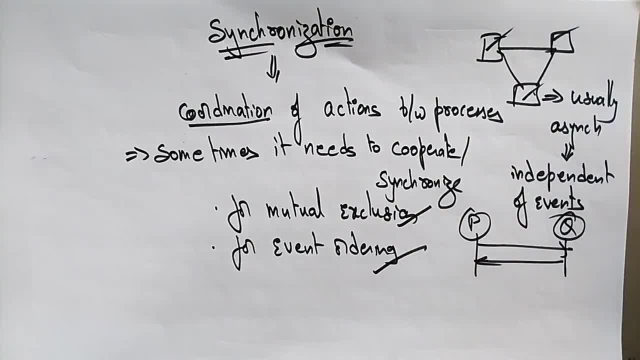 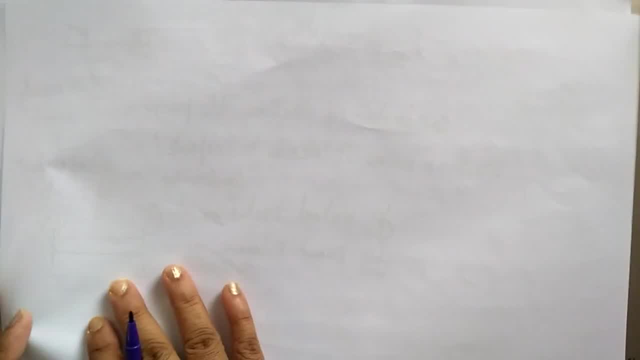 the synchronization in centralized- let me take a centralized distribution system and the sorry centralized system- and the distributed system. So now we are talking about the distributed system, a synchronization in distributed system only. but you have to know what. what is the role that is playing in centralization and in the distribution? 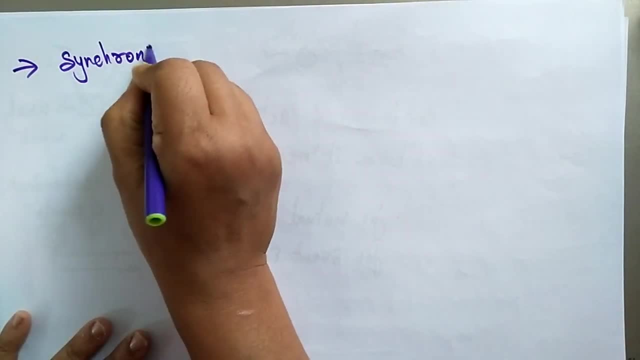 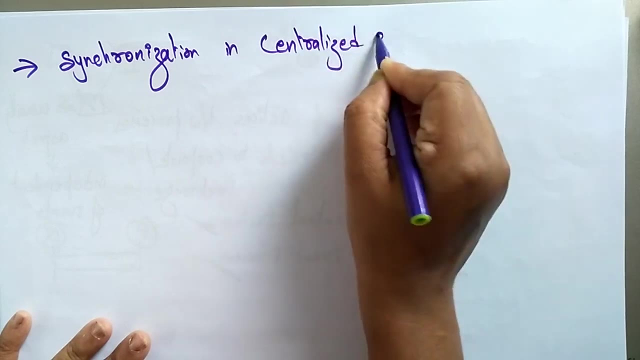 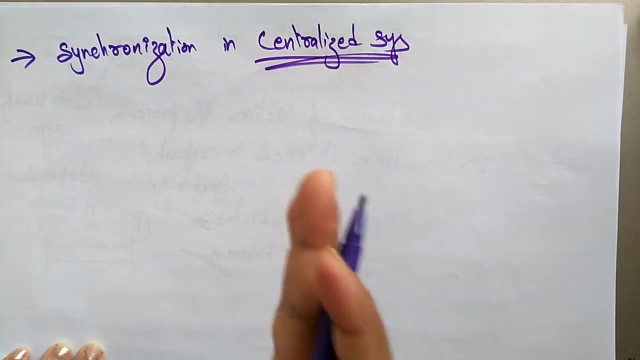 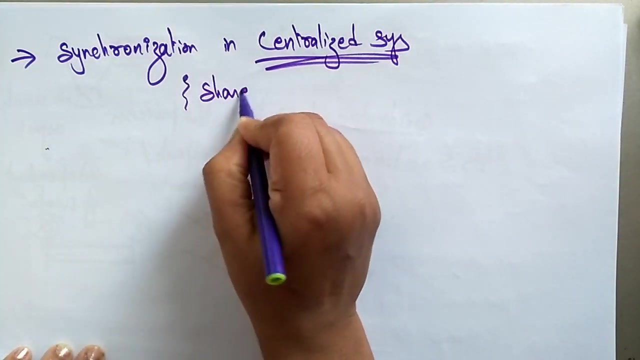 Okay, suppose, if you take the synchronization, synchronization in centralized system, not in distributed system- remember that it is a centralized system. so let us take a synchronization in centralized system. so here in centralized system, is primarily accomplished through shared memory. so here we use the concept shared memory. so if you are using the shared memory, 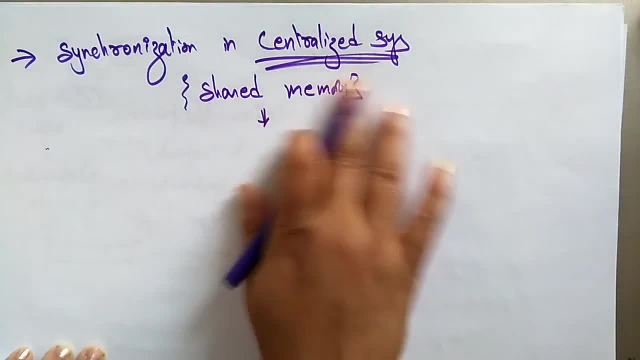 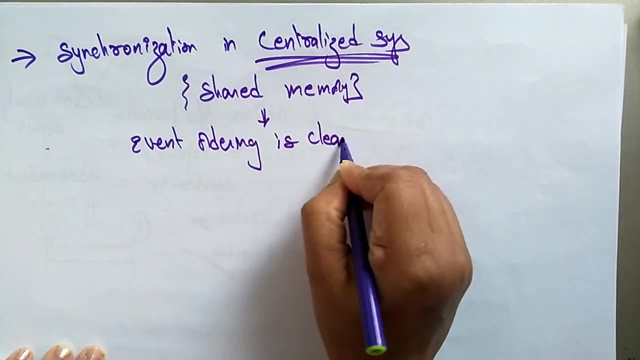 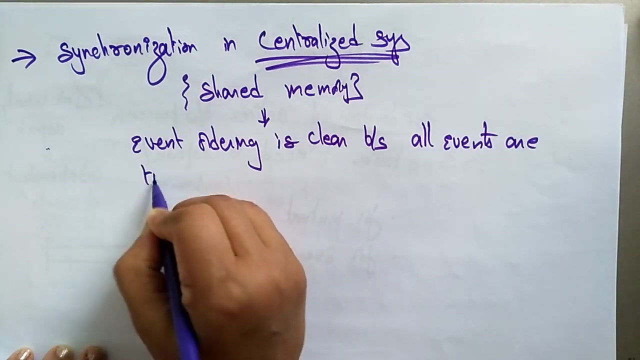 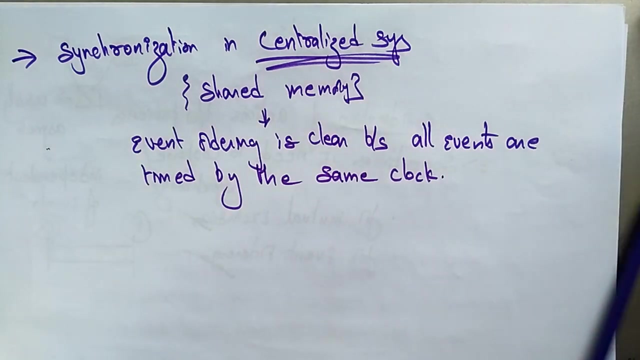 then the event ordering is clear. here event ordering is clear because all events or timed by the same clock, time by the same clock. so did you see what it is saying? so here how the synchronization is playing role in the centralized system. so in fact, the synchronization is playing role in the centralized system. so if you are using 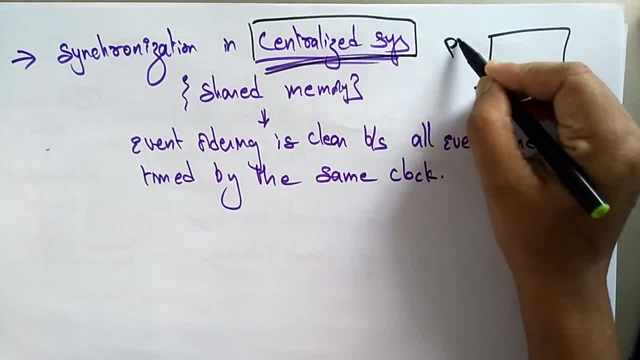 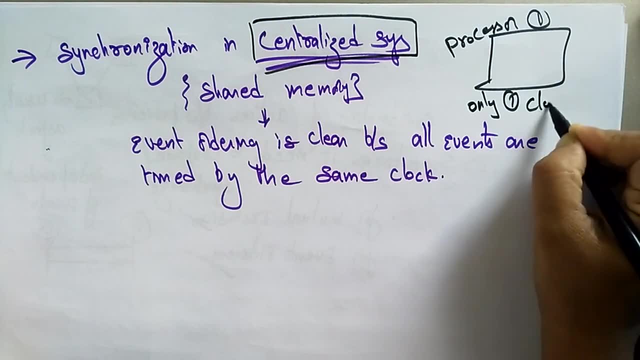 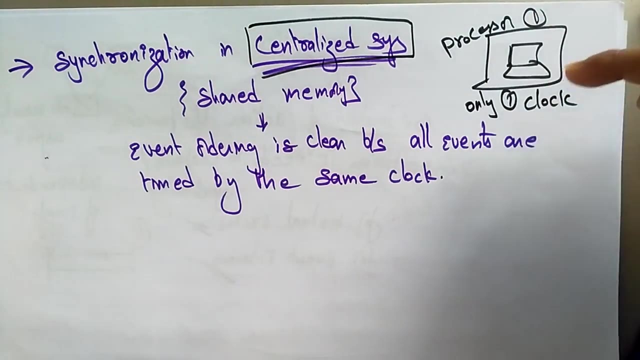 the centralized system means you are having only one processor, only one processor and only one clock, only one clock in the system. so this is a centralized system. in a centralized system, you are having only one processor and one clock. so here a memory is shared by all the process. so 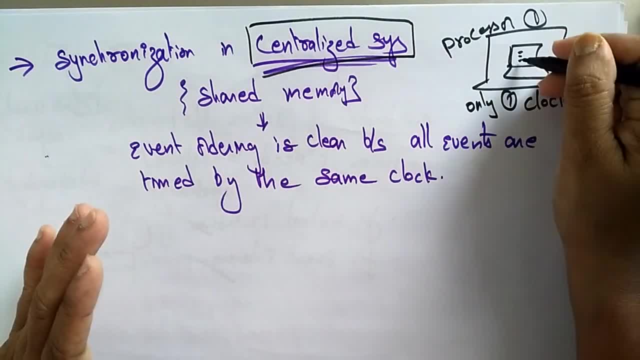 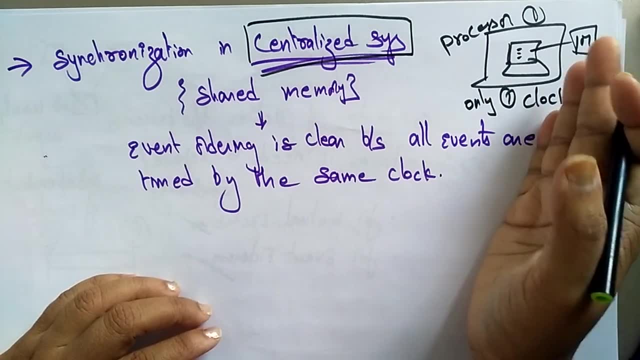 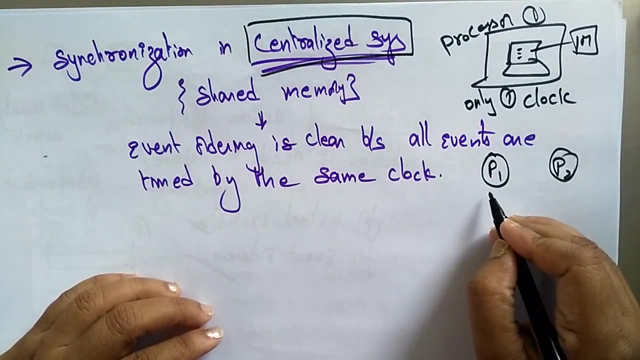 different process are executing in the system. so these process are sharing the same memory. okay, they are sharing, sharing the same memory. so here the event ordering is clear. so whenever one process is handling p1, another process will take p2, because p1 is already handled by the 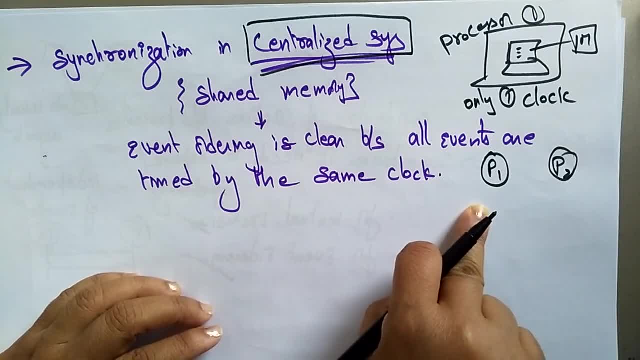 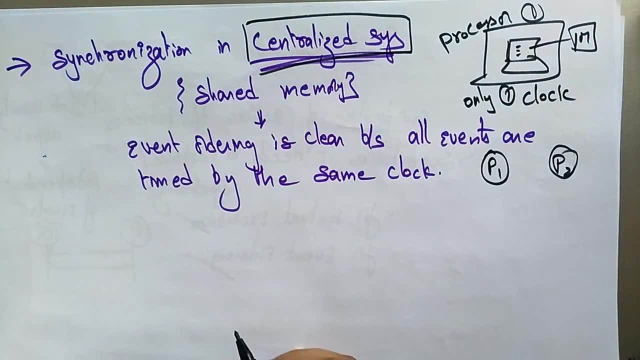 one is handled by another process how it knows, because everything is stored in the memory. these memory is shared by the process system. okay, so in the centralized system there is a shared memory. so shared memory is there. means each and every Тоfredi's memory is shared by P1 etc. 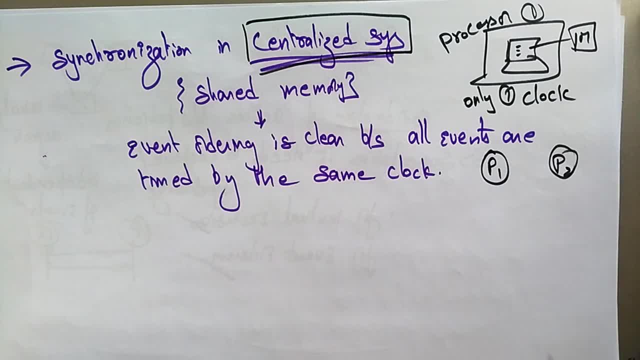 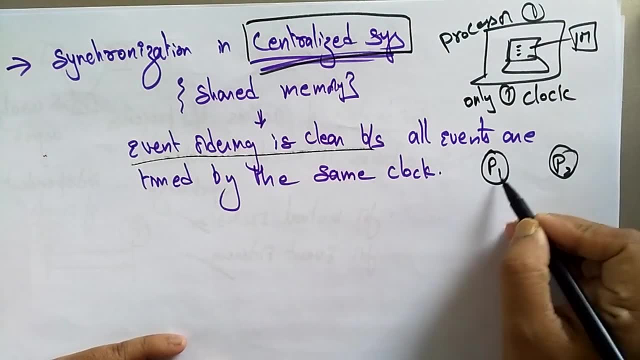 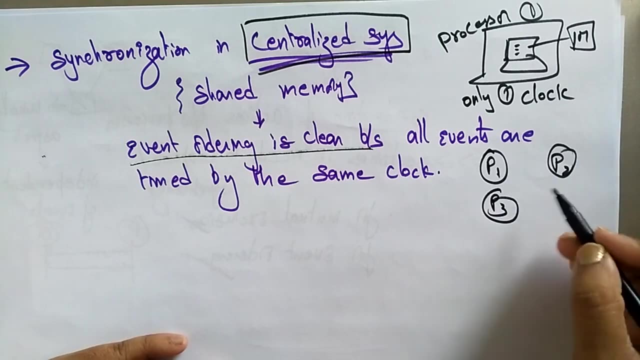 every process is able to see is whether the that process, a processor, is busy or not. so here the event ordering is clear. so one is assigned one. process is assigned one. another process is assigned two. another process is assigned three. suppose p1 time is over, so again, if it is, release the process. 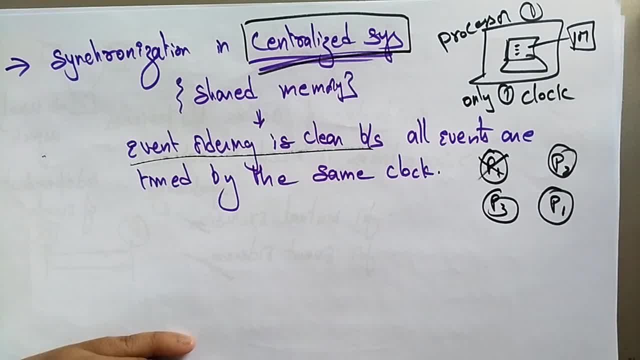 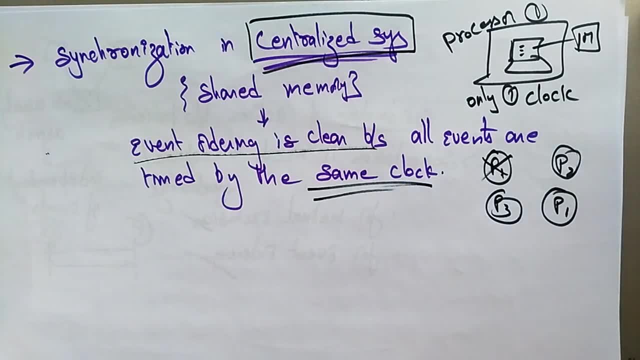 then again p1 will be, as one will be assigned to another processor, so all events are timed by the same clock. so that is the synchronization in centralized system. so here, if you observe, event ordering is clear, so that all the events are timed by the same clock. 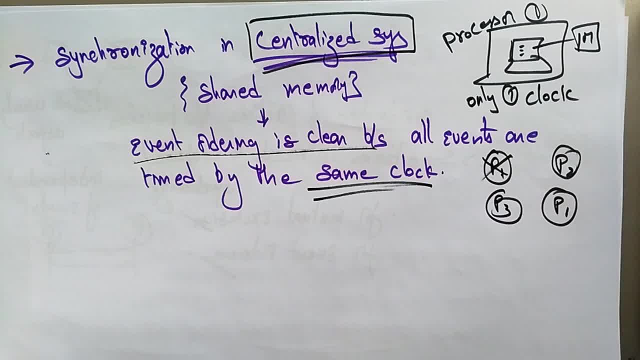 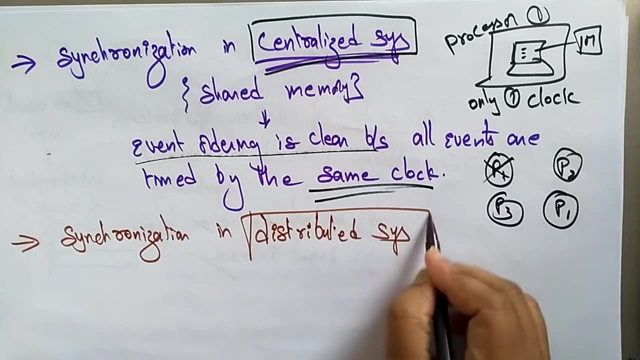 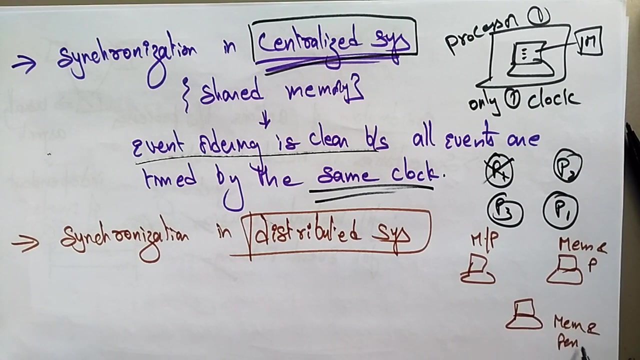 then coming to the asynchronous- sorry, synchronization in distributed system. synchronization in distributed system. so distributed system means so many systems are there, so many systems are there, each system is having their own memory and processor, own memory and processor, each system having their own memory and the processor. so here in the synchronization, uh, synchronization in distributed system is harder. 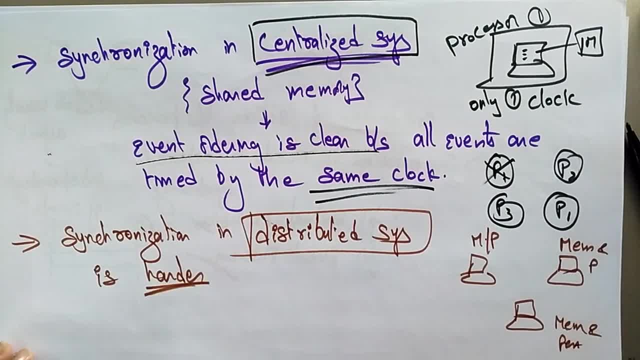 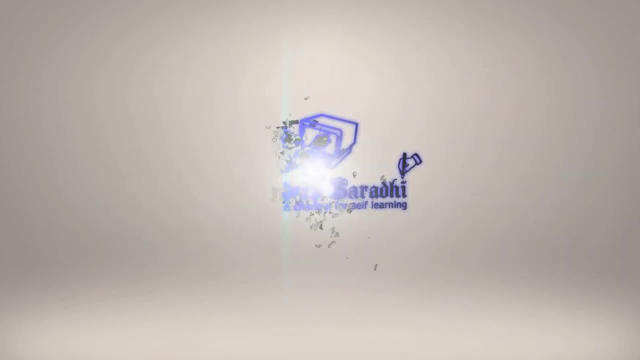 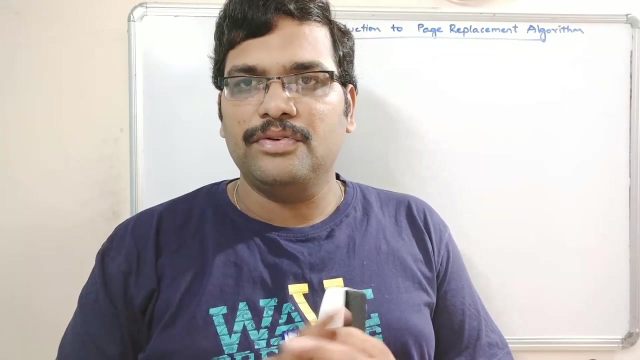 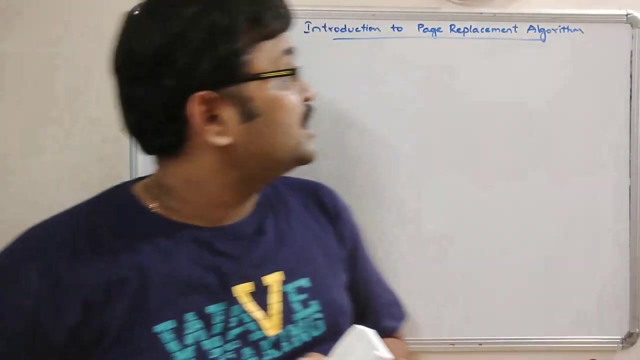 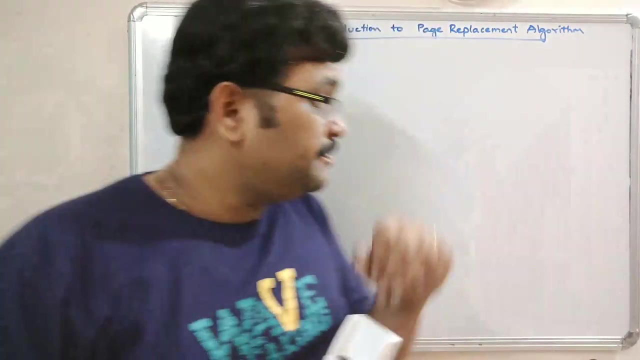 hello friends, welcome back to our channel. so hope all are doing well and safe at home. so don't go outside and stay at home and be safe, right. so today we are going to discuss about one more concept in operating systems, that is, page replacement algorithms. so in that we will. 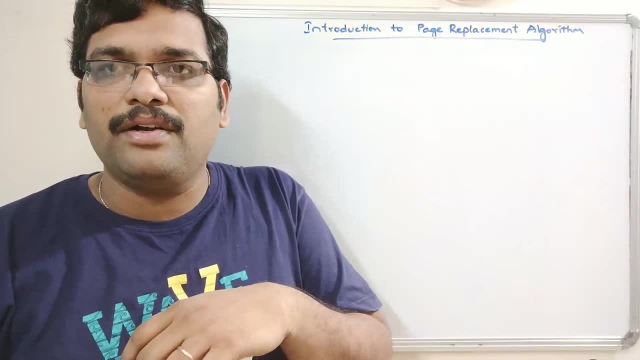 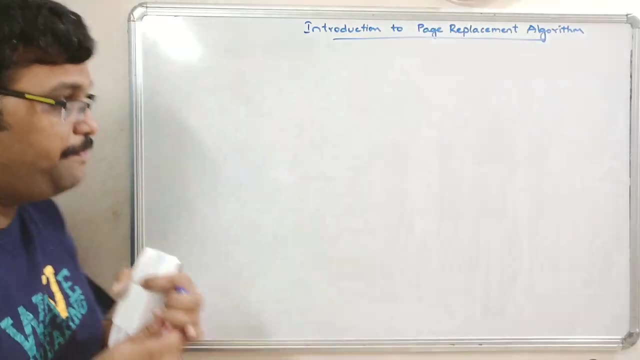 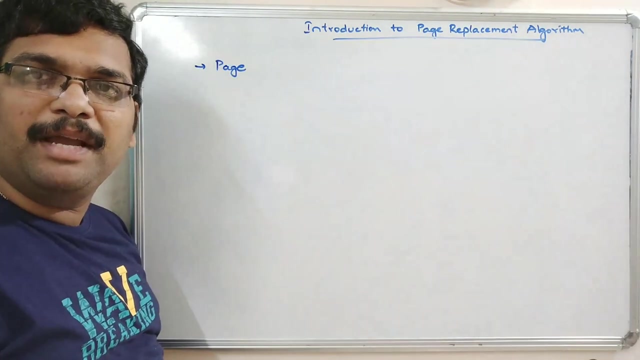 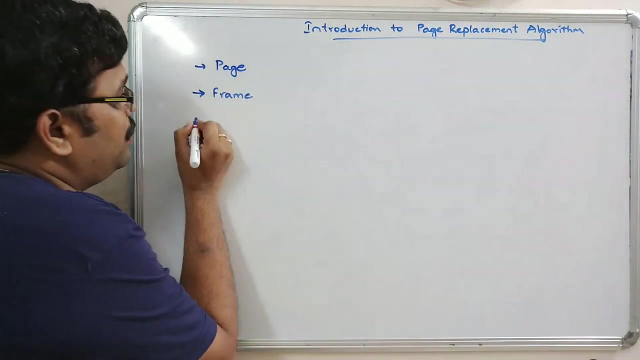 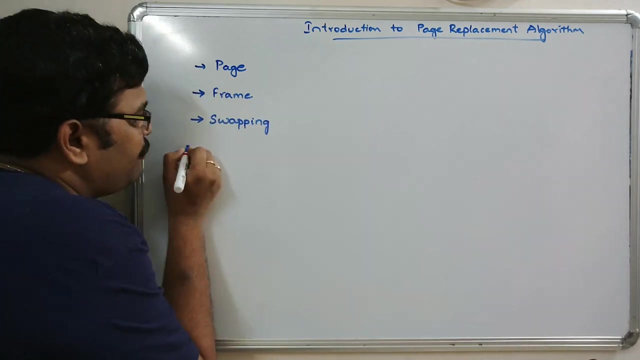 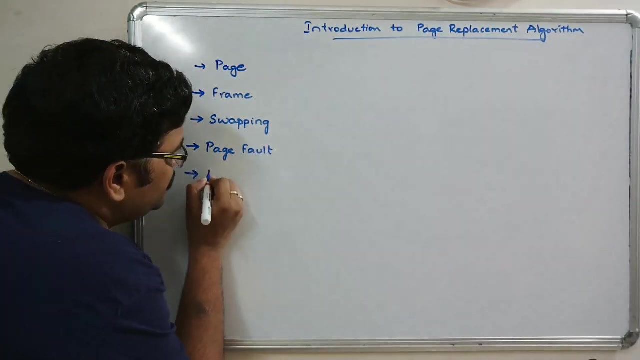 see what are the basic terminologies we are required to know before going to this page replacement algorithms. so the basic terminology is used. the first one is page, so what is meant by a page? second one is frame. third one is swapping. fourth one is page font. fifth one is hint. next one is the techniques.